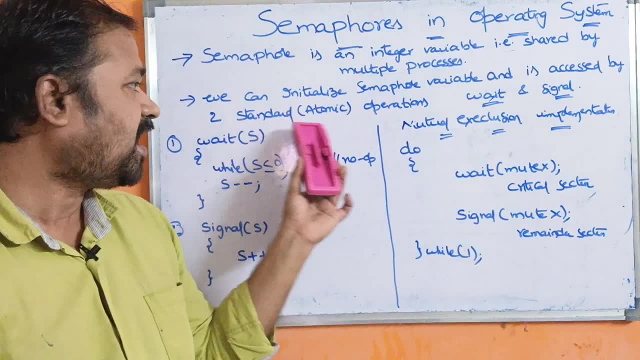 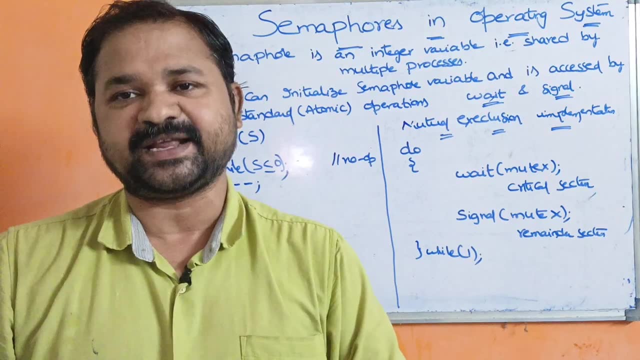 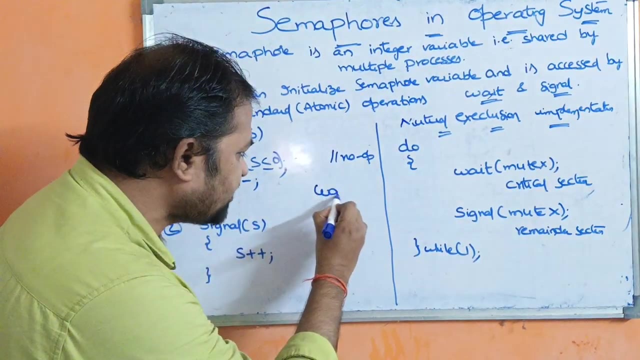 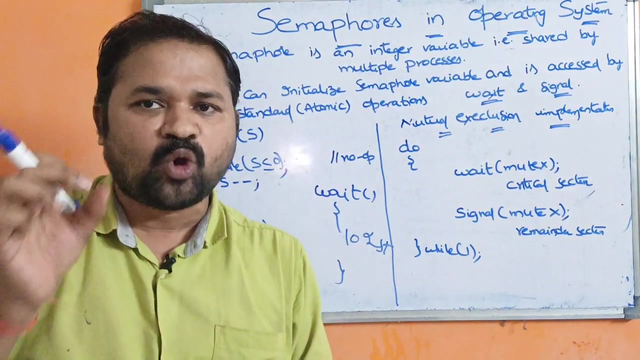 mainly performs two standard operations. They are weight and signal. Here weight and signal operations are called as atomic operations. Atomic operation means: let us assume that weight function contains, let us assume that weight function contains 10 instructions. So when a process is executing weight operation, then we must execute. 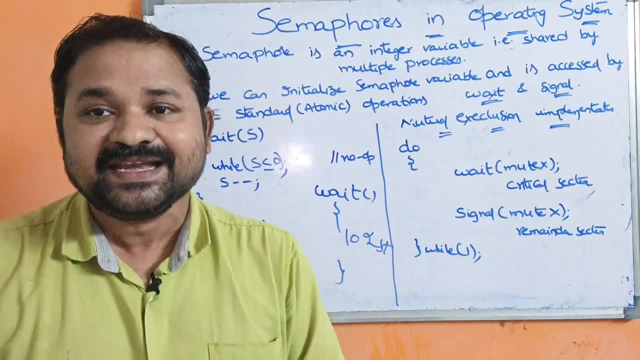 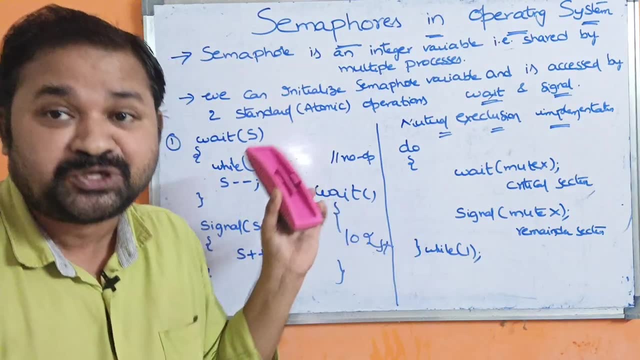 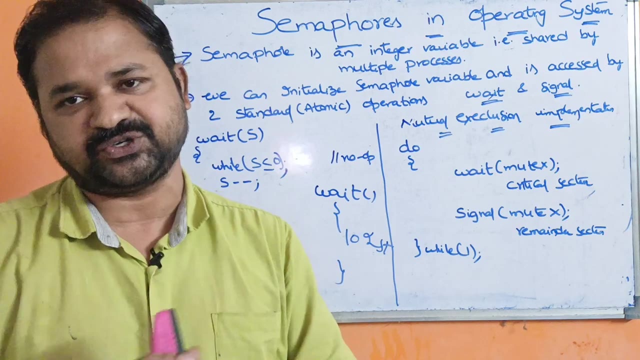 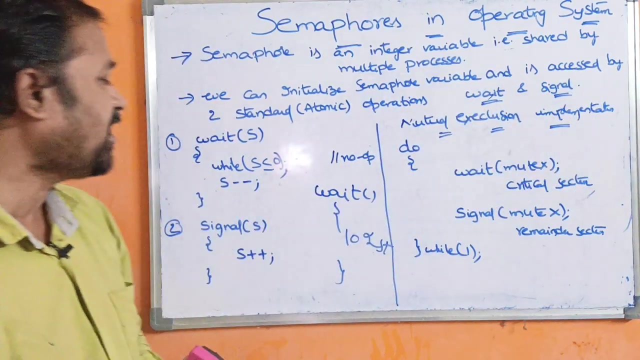 all the 10 instructions In the middle. it is not possible to forcibly stop this function. It is not possible to interrupt this function. So all the instructions in that function should be executed, must and should. So that is called as atomic atomic. Okay, now let us see about weight and signal operation. So weight of yes, yes, means semaphore variable. 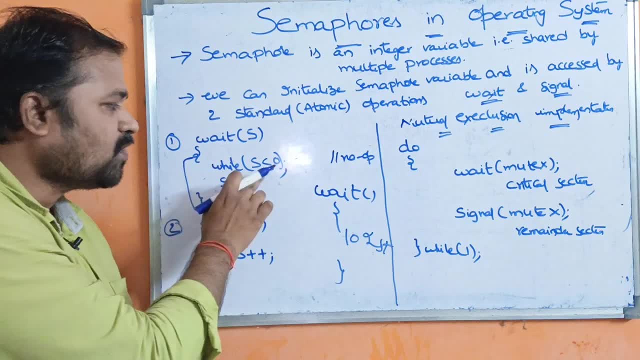 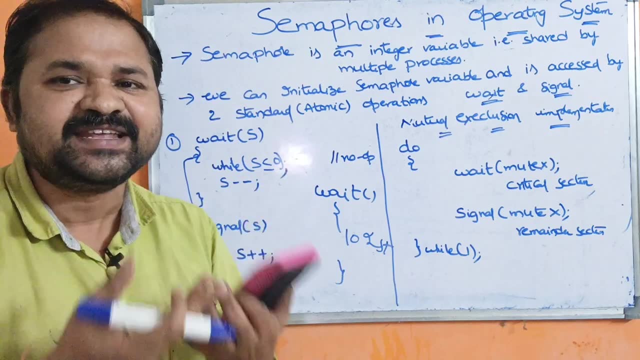 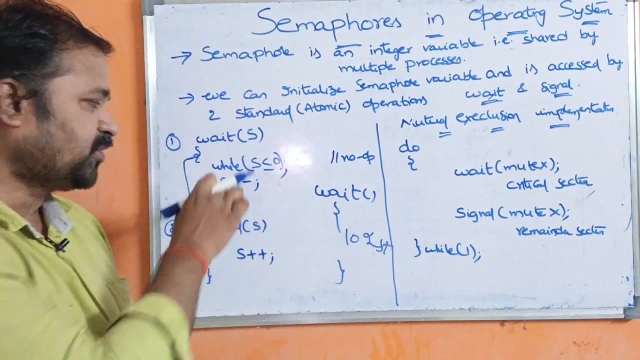 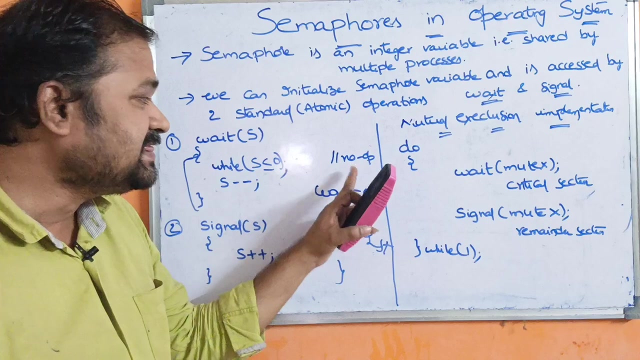 Let's see the code for weight. So weight of yes, while yes is less than or equal to 0 semicolon. That means we know that we can initialize the semaphore variable. So initially we have to check the value of the semaphore variable. If yes is, while yes is less than 0 or while yes is is equal to 0, then there is no need to perform any operation. That process will be in weight and signal operation. 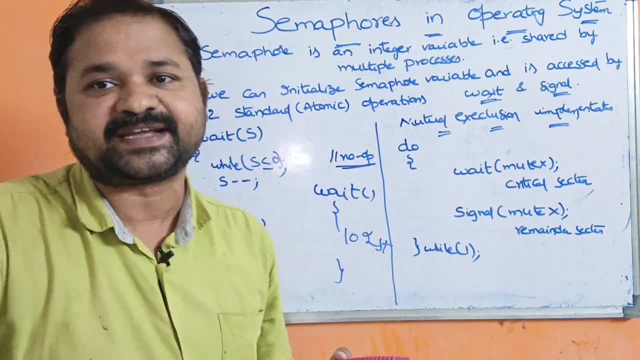 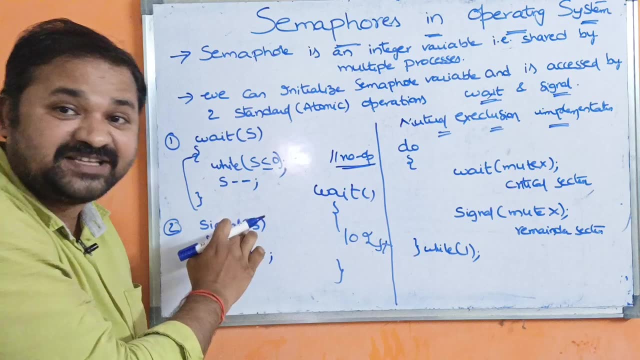 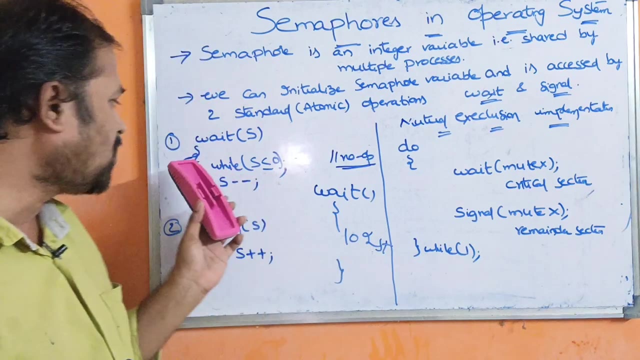 state that process will be in blocked state, sleeping state. suppose while s is greater than 0. while s is greater than 0, then we can decrement the value of the semaphore by 1. so this is the logic for weight operation. so here we have two conditions, are there? first condition is: if s is 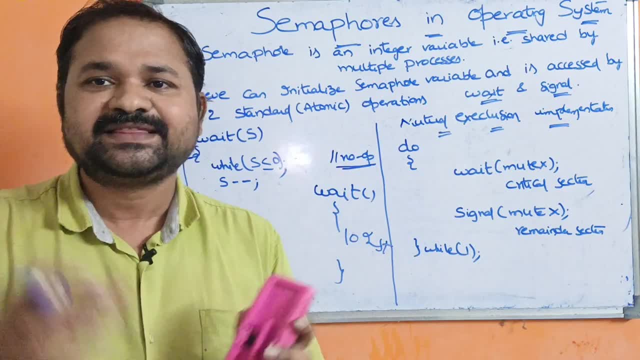 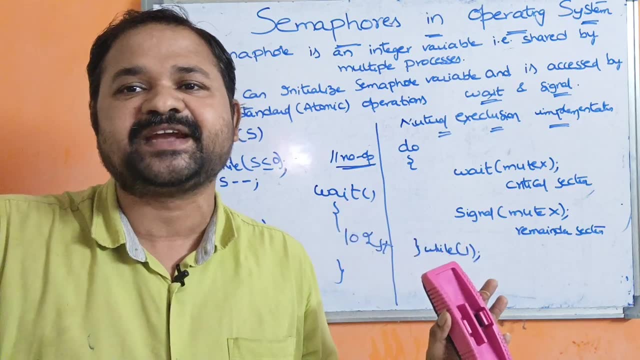 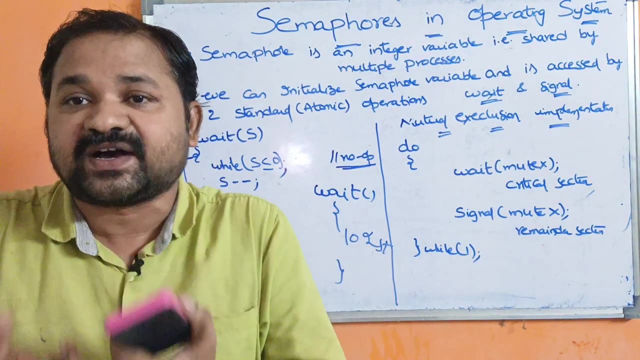 less than 0 or s is equals to 0, then do nothing. there is no need to perform any operation. that process will be in sleeping state or some blocked state. otherwise suppose. if s is greater than 0, that means if semaphore variable contains a positive number. it may be 1 or 2 or 3 or 4. 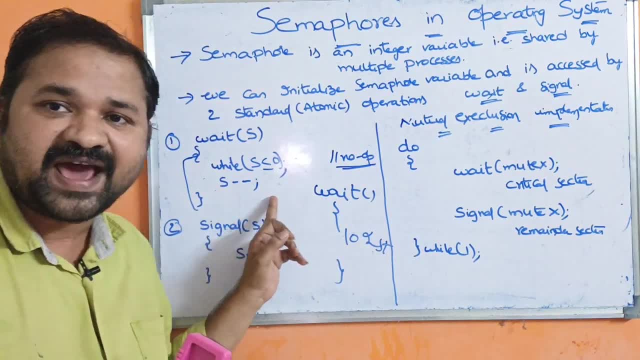 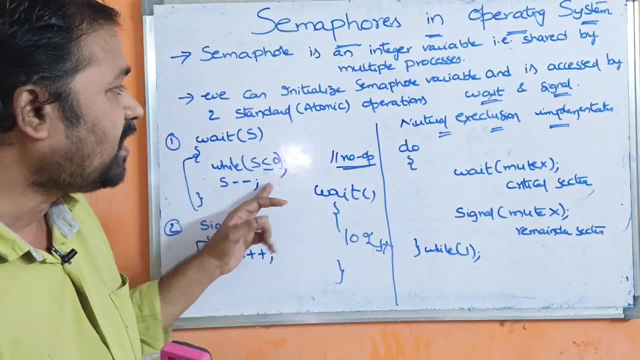 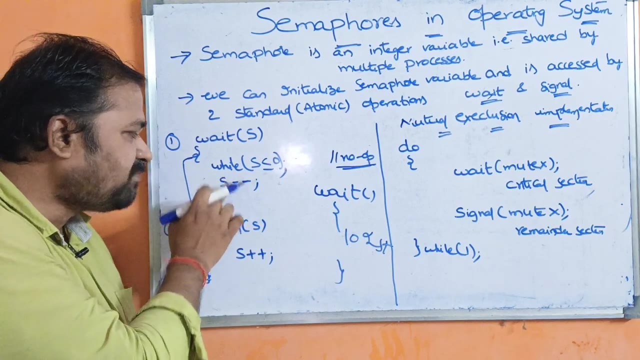 any positive number, then we have to decrement the value of the semaphore by 1. okay, now let us see how to decrement the value of the semaphore by 1. about the second operation, that is, signal operation: here already i said that these two operations are atomic operations if you take a weight weight. here we have two statements are: 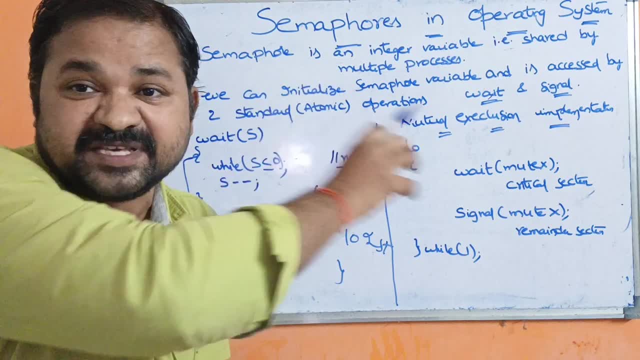 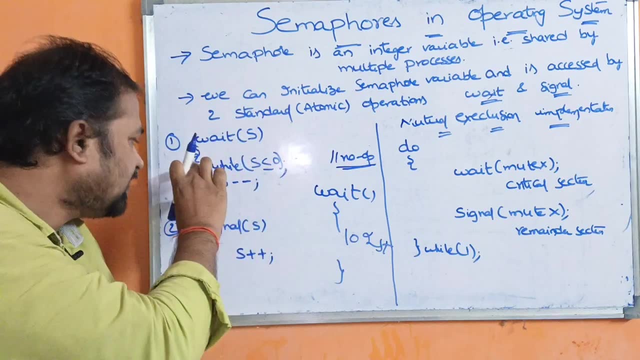 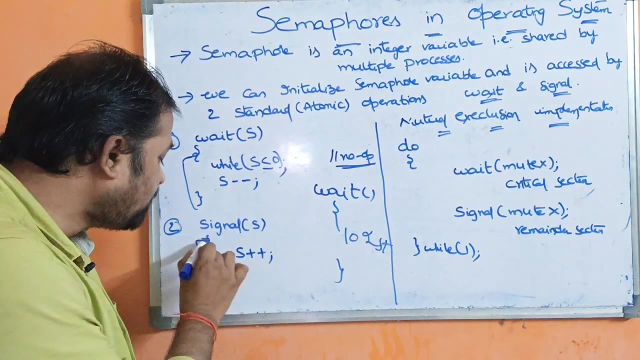 there. so it is not possible to stop this function when the process is executing the first two statement. we must and should execute the two instructions in the weight function. okay, that's why this is called as atomic operation. now let us see about signal operation. signal operation, signal of- yes, that means we are performing signal operation on the semaphore. 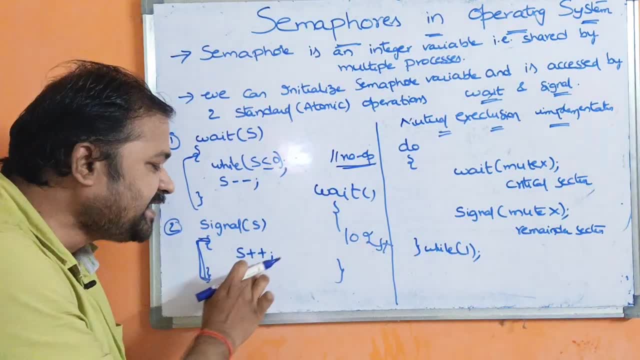 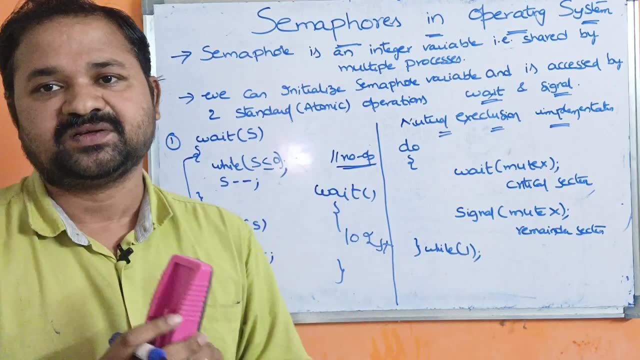 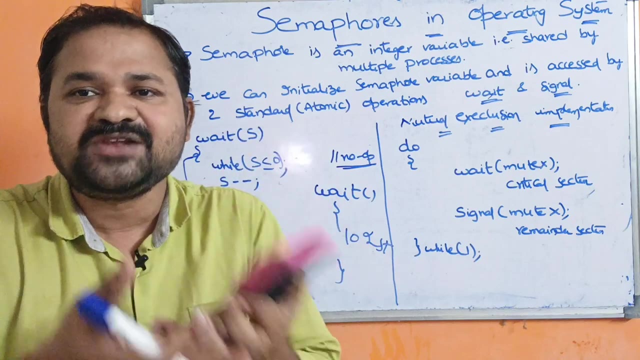 variable. here simply we have to increment the value of the semaphore by 1. so in signal operation there is no need to check any condition. simply here we have only one statement is there, that is s plus plus. that means increment the value of the semaphore by 1. here semaphores are mainly useful. 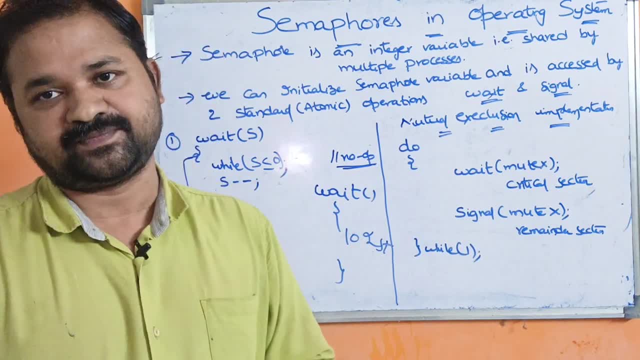 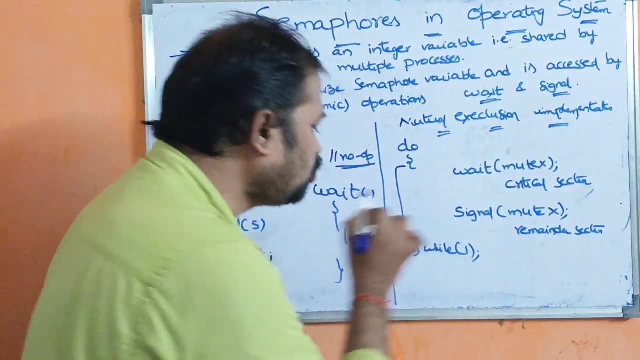 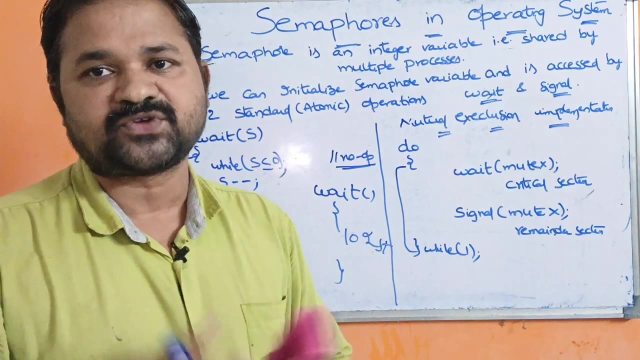 in order to implement the value of the semaphore by 1. so in signal operation there is no need to mutual exclusion. let us see how we can implement mutual exclusion here. this is the code here: do while of one semicolon, so one specifies that this condition is always true. so one means true, zero. 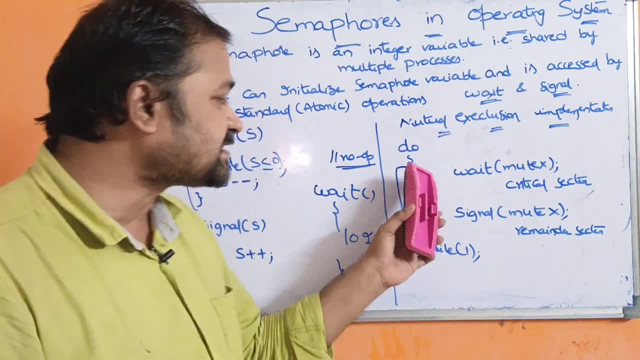 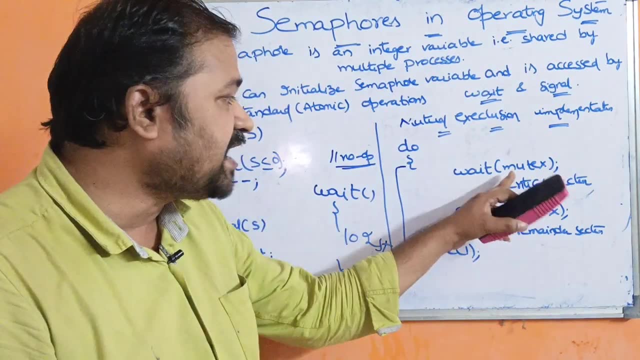 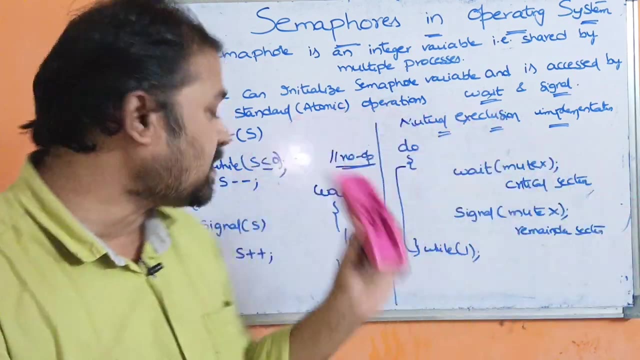 means false. so while of one semicolon so one means this condition is always true. so what is the first statement here? in order to implement the mutual exclusion, we are taking a variable called mutex, where mutex stands for mutual exclusion. here mutex is nothing but semaphore. variable value. 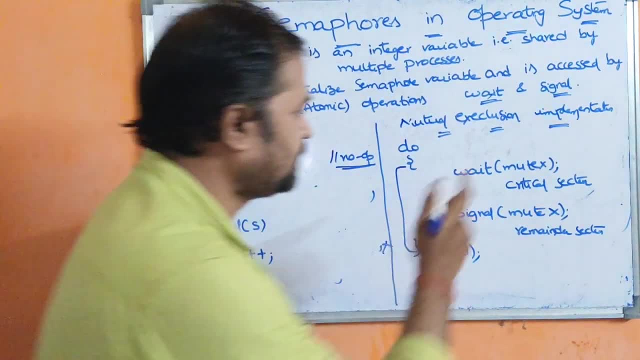 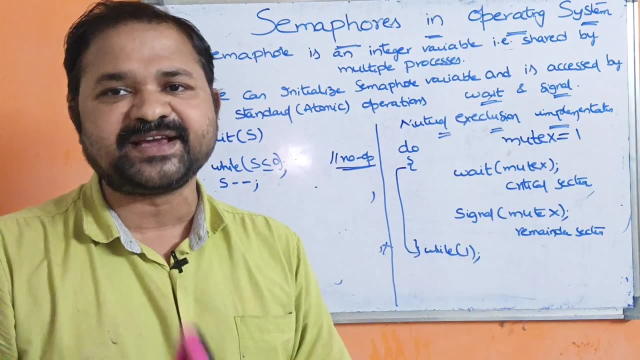 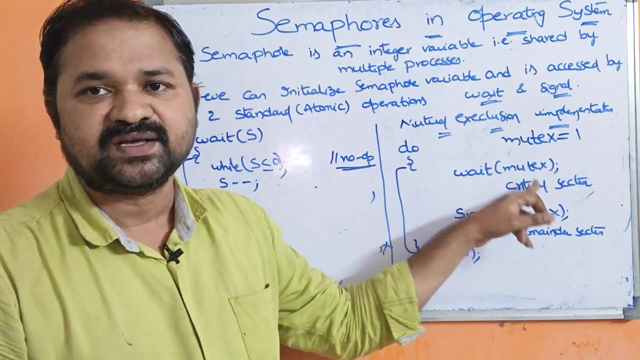 here the initial value of the mutex is one. so we know that we can initialize the semaphore variable value let. the initial value of the mutex is one, so first we have to execute weight of mutex. so what is mutex value one. so first we have to execute weight operation. 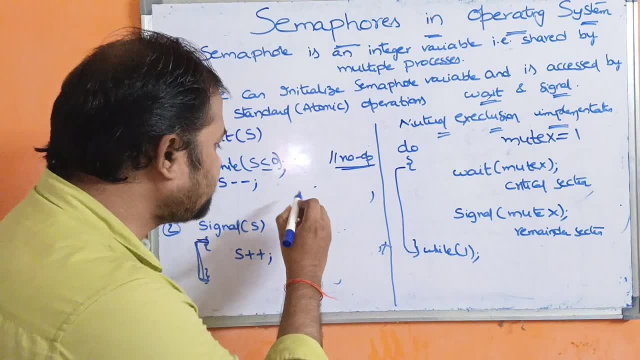 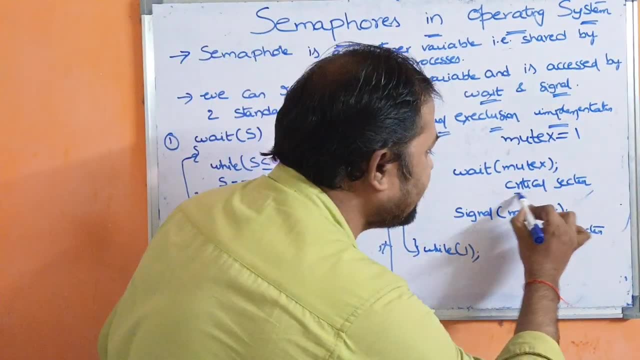 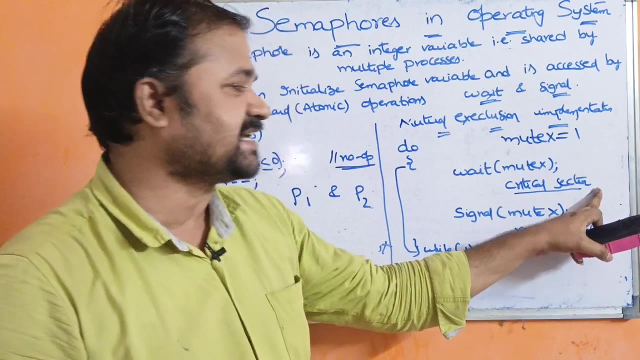 let us assume that two processes, such as p1 and p2, wants to enter into the critical section. so here we have critical section, is there? so? weight of mutex semicolon: if this condition is true, then the process can enters into the critical section. if this condition is true, then this process can enters into the 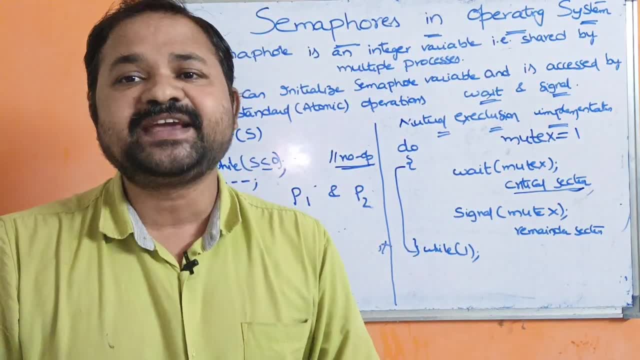 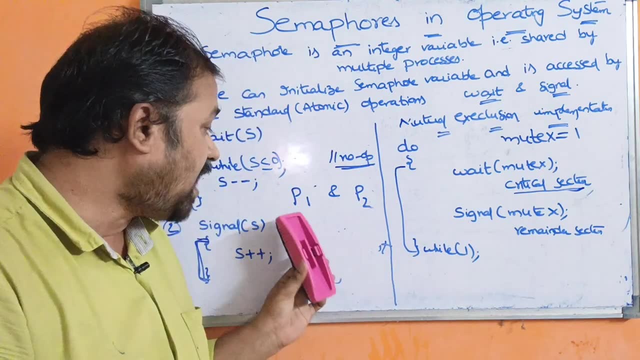 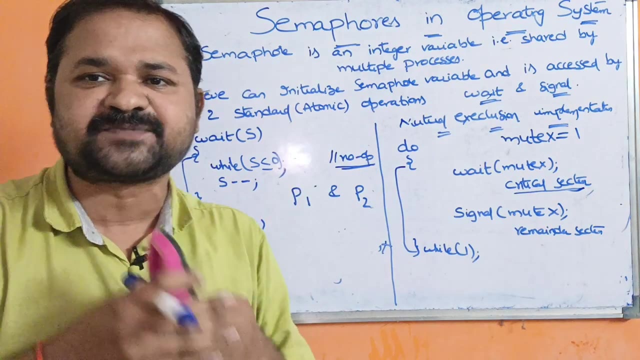 critical section. okay, so what is a critical section? so critical section is a part of the program where the shared memory is accessed. here we have two processes. are there p1 and p2? in critical section, the two processes, such as p1 and p2, can access the shared memory. 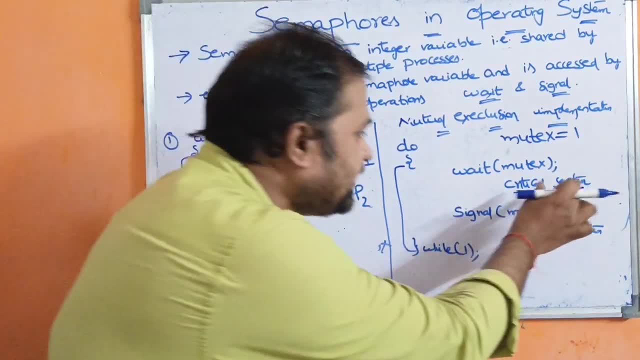 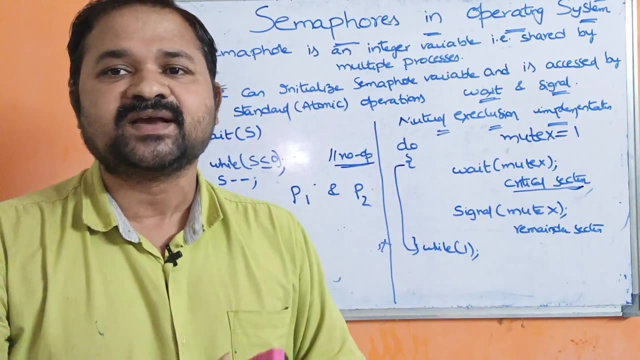 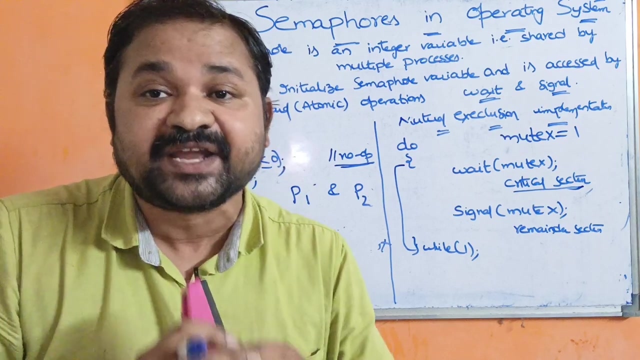 such as mutex. here in this critical section only the shared memory is accessable. the shared variable will be accessible here. the constraint is when one process is in the critical section, then no other process is allowed to enter into the critical section. when p1 process is in critical section, then it should have learned from the other process. 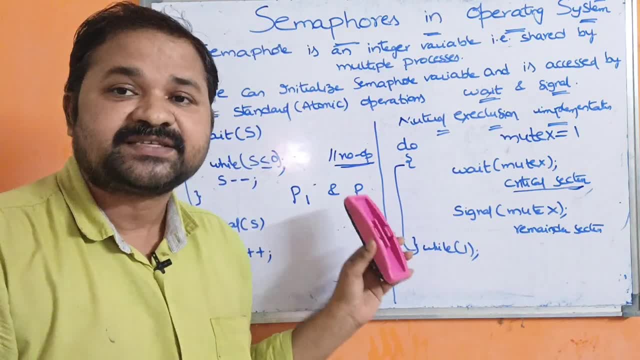 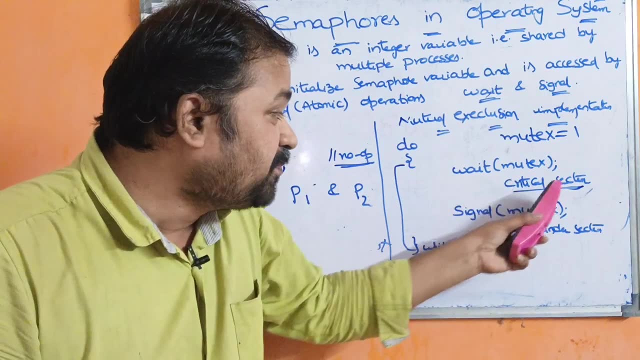 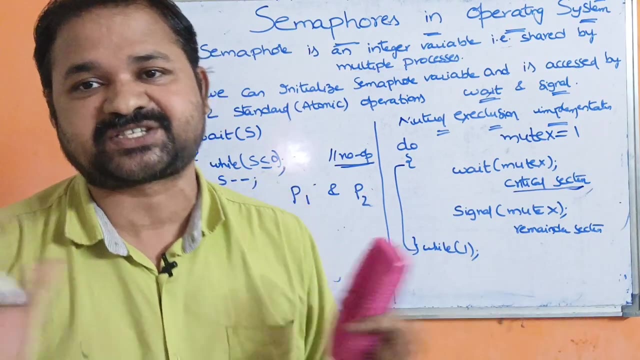 is in the critical section, then other processes, such as p2 and p3, are not allowed to enter into the critical section. why? because when multiple processes access the shared variable simultaneously, then it leads to wrong results. so that's why only one process should be in the critical section. 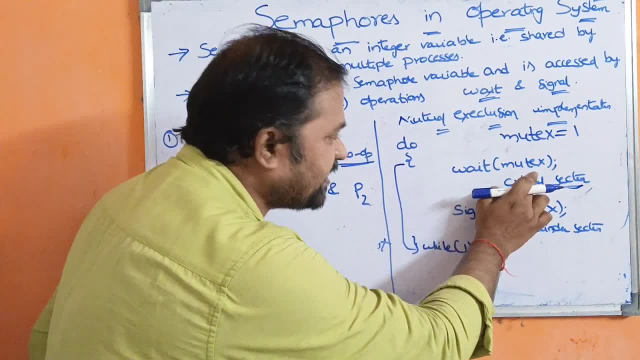 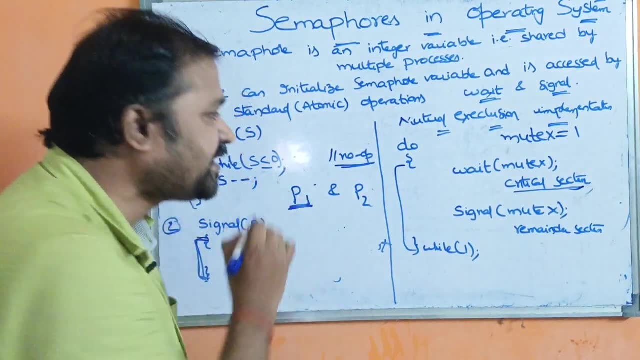 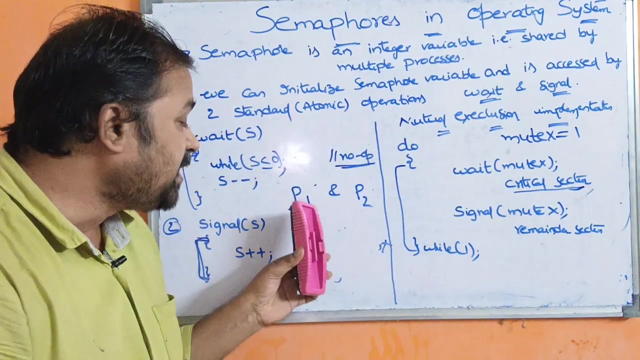 now let us execute weight operation, weight of mutex. so what is the value of the mutex one? so now let us assume that p1 process executed weight operation first. here two processes are willing to enter into the critical section. assumes that p1 process has executed weight operation. 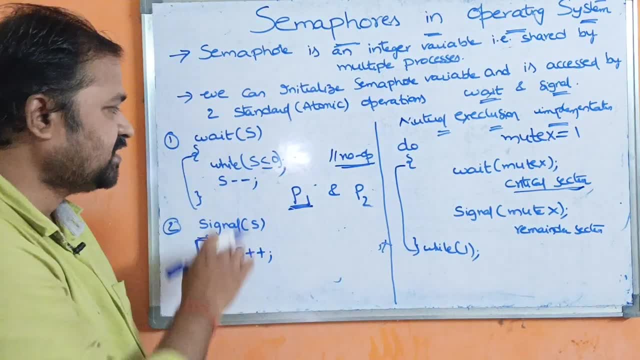 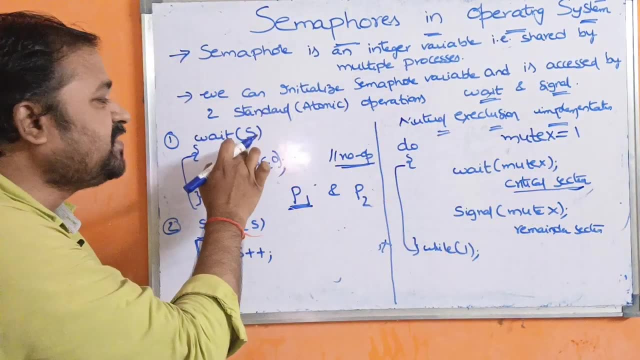 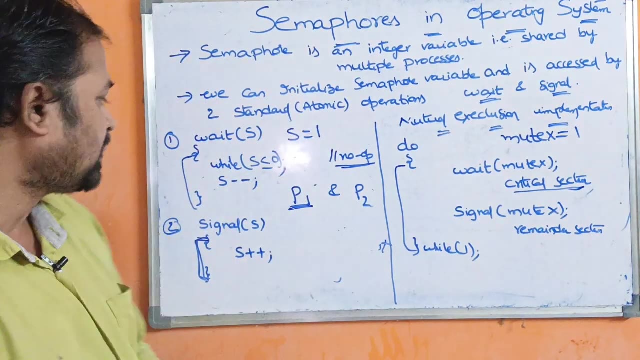 first, so now the control goes to the weight operation. so what is the value of the initial value of the? yes, what is the initial value of the mutex one, so that one will be passed to yes. so now, what is s value? what is s value? you one now, yes, value is one, while yes is less than or equal to zero. so one is less than or equal to. 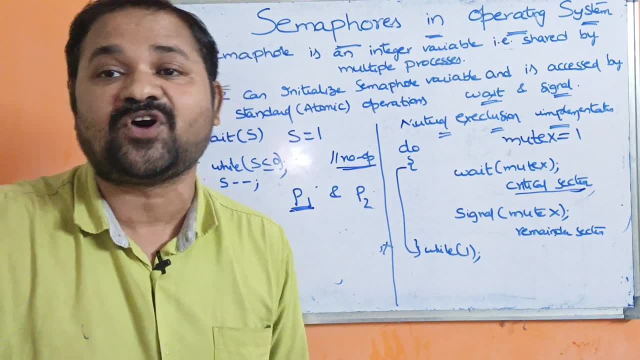 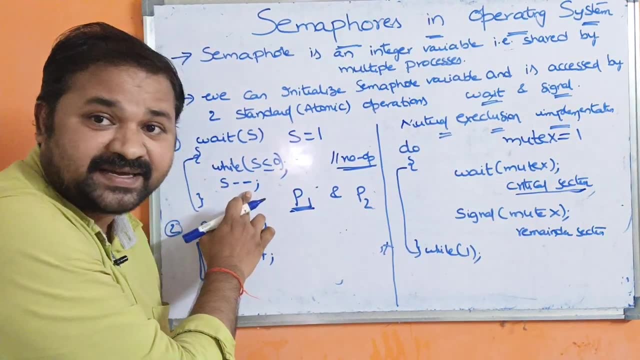 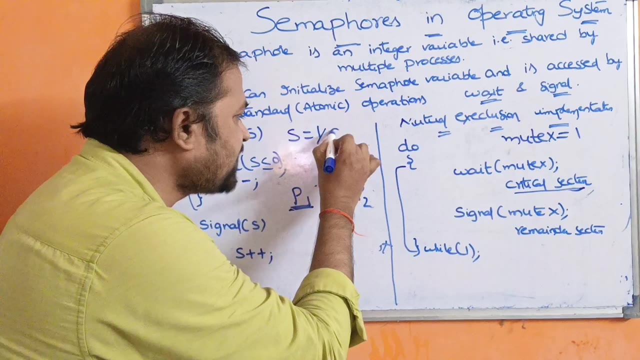 zero. one is less than or equal to zero condition is false. that means m4 is a positive value. if it is a positive value, then what we have to do, we have to decrement yes by one. what is the initial value of the yes one? so one minus one means zero. now, yes, value is zero s value is zero. so p1 process. 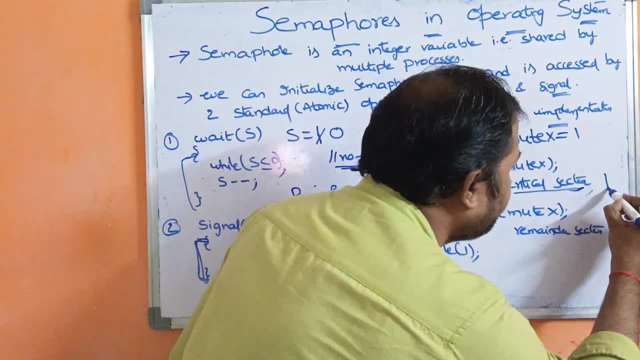 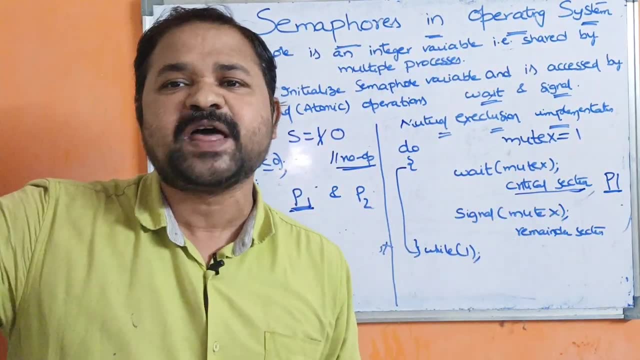 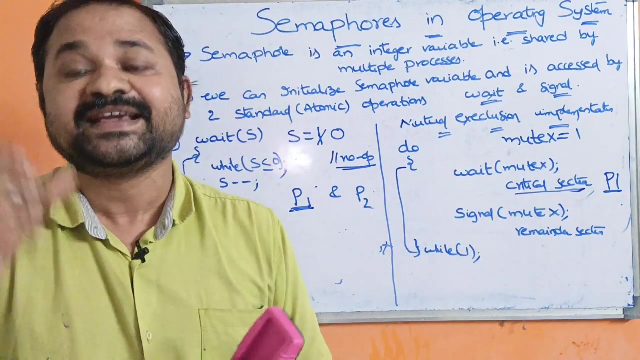 enters into the critical section now. now assumes that p1 process is in the critical section. when p1 process is in the critical section, then no other processes are allowed to enter into the critical section. so let us assume that p1 is in the critical section and in the meantime assumes: 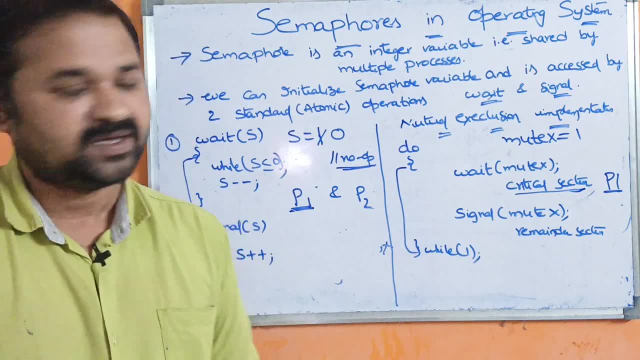 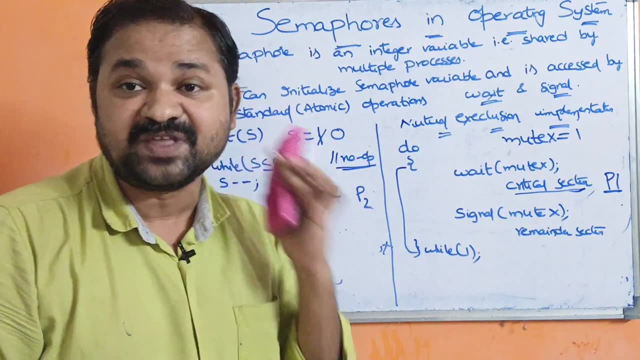 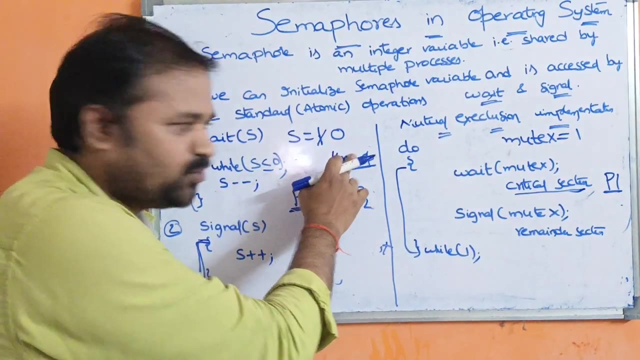 that p2 is trying to enter into the critical section, so for that, p2 executes weight operation one more time. now what is the value of the mutex? what is the value of the mutex previously? its value is one only, but after that it is changed to zero. after that it is changed to zero. now, what is? 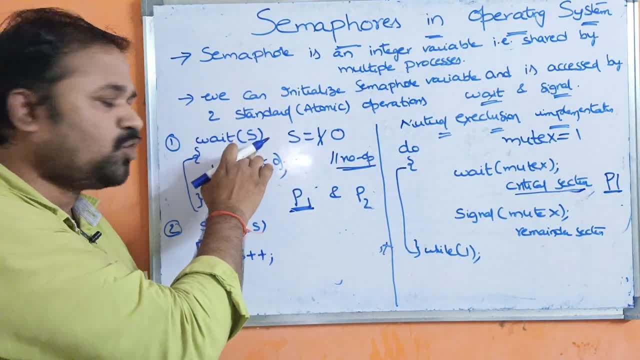 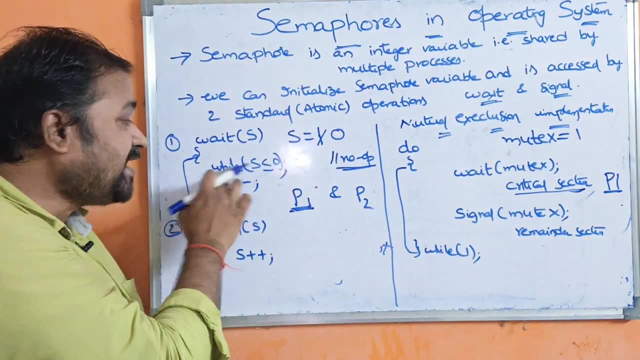 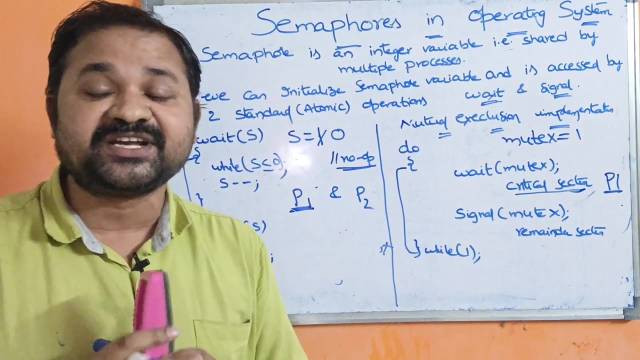 mutex value: zero, zero. so now control goes to the weight function. now s value is: what is s value? what is s value? zero? s value is zero, now, while of s less than or equal to zero. zero is less than or equal to zero. zero is less than or equal to zero. condition is true, so p2 process cannot enters. 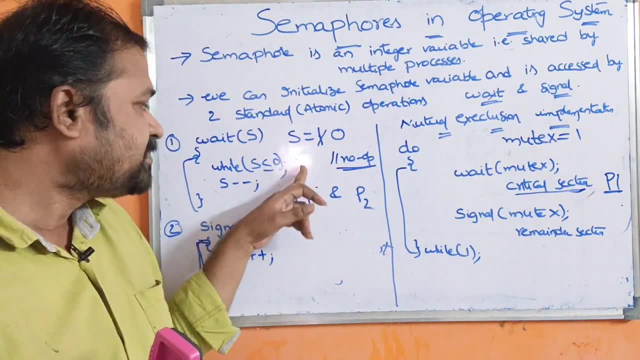 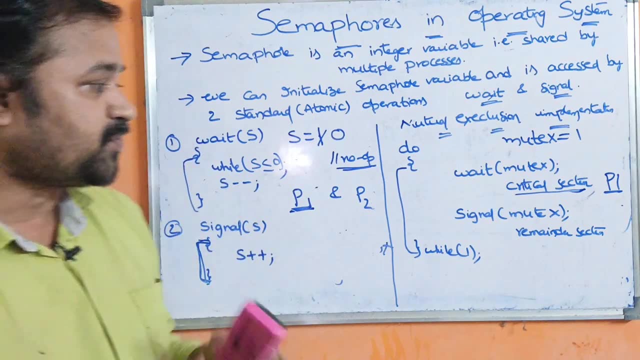 into the critical section. if the condition is true, then that process has to be weight. okay, so p2 process is not allowed to enter into the critical section. so when p2 process can enters into the critical section, let us see that code now. okay, so here p1 process is in the critical. 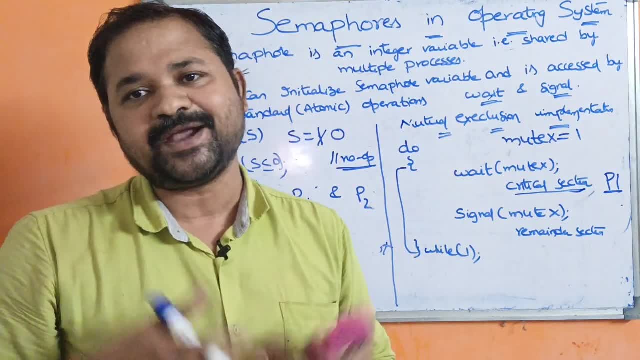 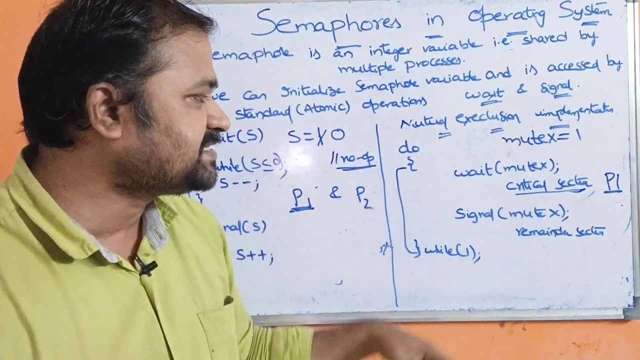 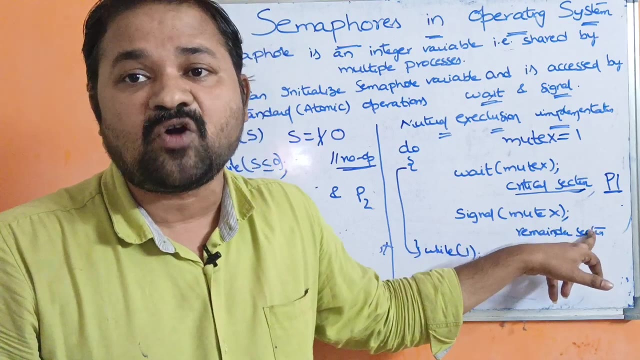 section. let us assume that p1 process has completed all its operations. so after that, p1 process comes out from the critical section, after coming out from the critical section, p1 process- execute signal operation. p1 process: execute signal operation. signal of mute x. so now the control goes. 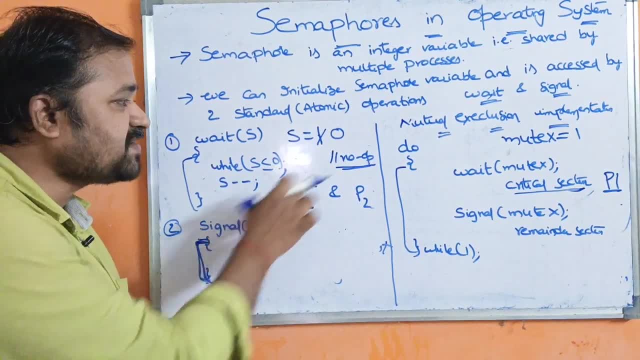 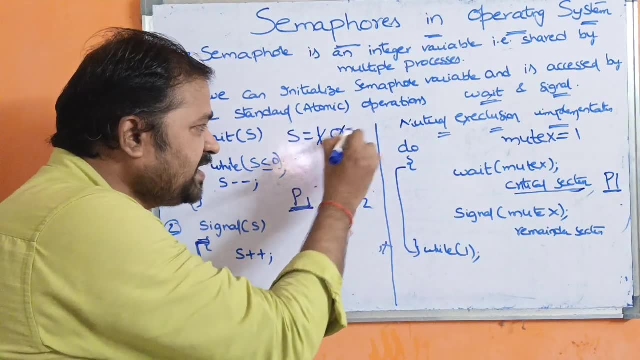 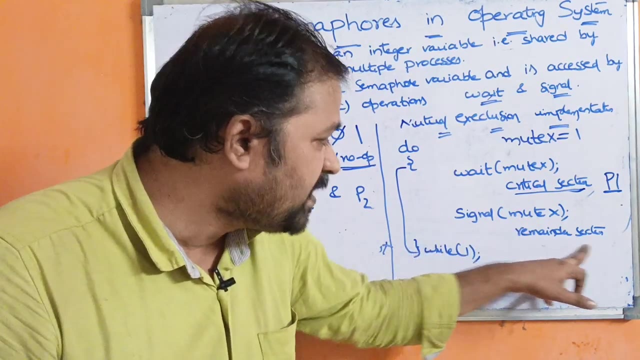 to the signal operation: signal operation. so what is the value of the s? what is the value of the s zero? what is signal operation s? plus, plus now, zero value will be incremented now. now s will become 1. okay, so after executing the signal operation now, p1 process will be in the remainder section. 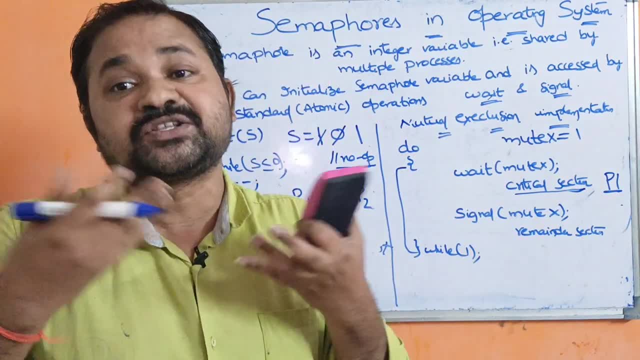 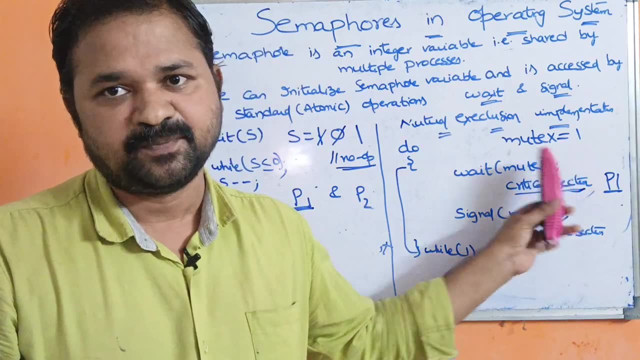 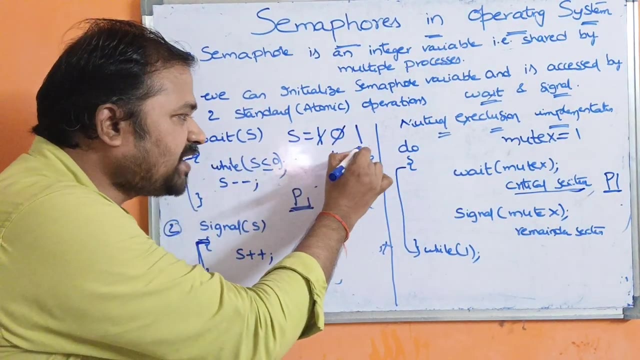 now assumes that p2 process wants to enter into the critical section. so now what the p2 process will do. p2 process execute weight operation. p2 process execute weight operation. so weight of mutex. so control goes to the weight operation, weight of s. so now what is s value, what is s? 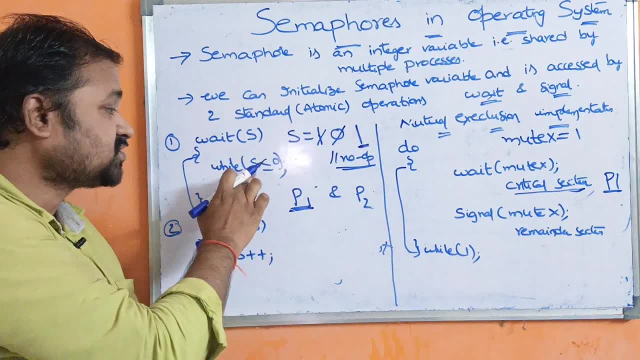 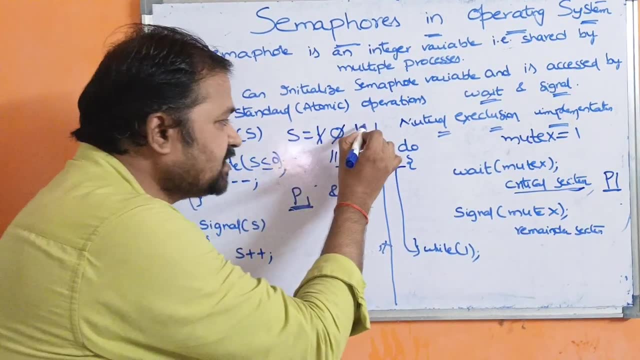 value. s value is 1, s value is 1, so 1 is less than or equal to 0. 1 is less than or equal to 0. condition is true. so yes, minus minus. so previously s value is 1, now yes, value will become 0, so p2.